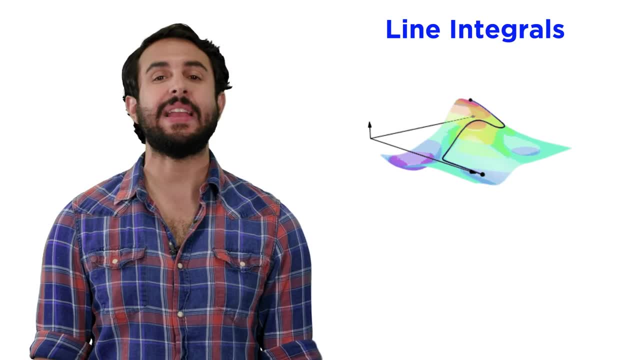 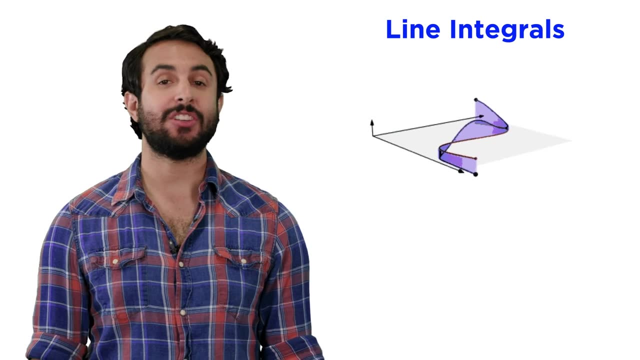 f of x- y. Now with line integrals we can integrate a surface f of x- y along the path of some curve C. We will be integrating along small segments of the curve C, which we will call ds. 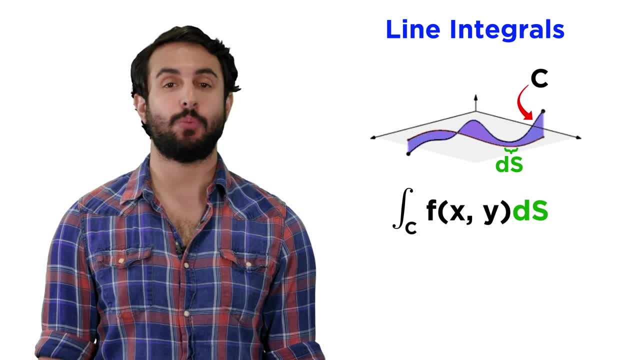 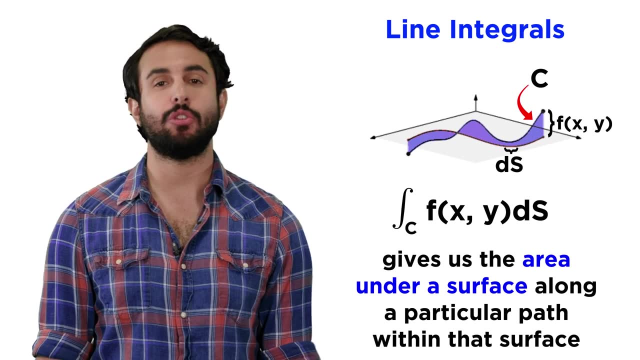 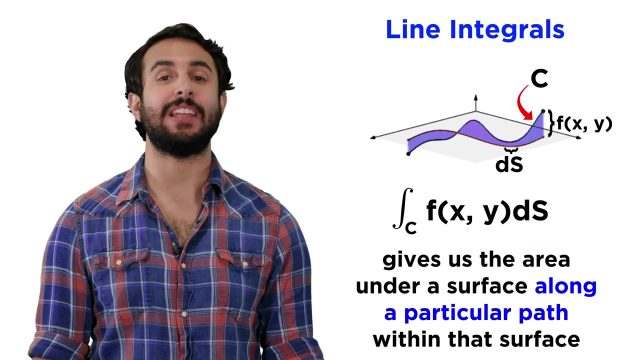 Just like when we initially learned integration, these segments will be our widths, while the surface f of x, y will be our heights. So, once again, our integration will give an area, but now we are finding the area that is under a surface, along a particular path within that surface. 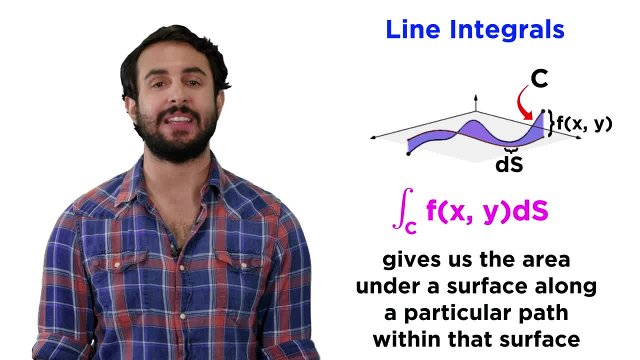 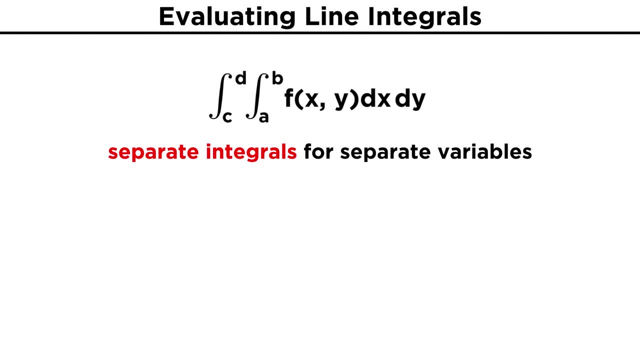 The way we will write this out is the integration along C of f of x, y, ds. Recall that when we learned how to evaluate multiple integrals, the x and y variables were treated independently during the integration, But now, with line integrals, we have a single integral with both x and y. We must keep in. 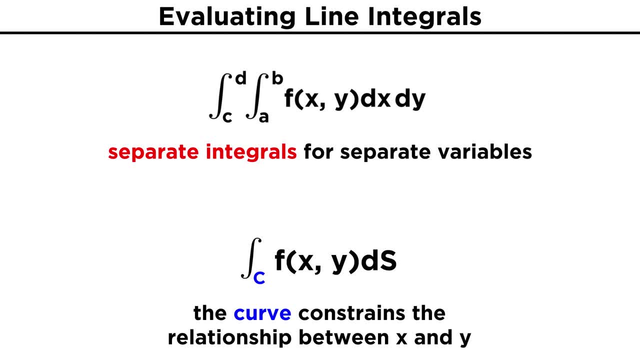 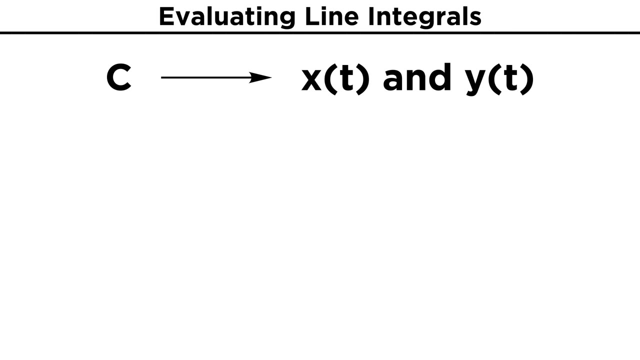 mind that the curve we are integrating along constrains the relationship between the two variables. Because of this, we can no longer treat them independently, but this also opens up the possibility of reducing things to a single variable that is to be integrated. In order to calculate line integrals by hand, it is often necessary to be able to express. 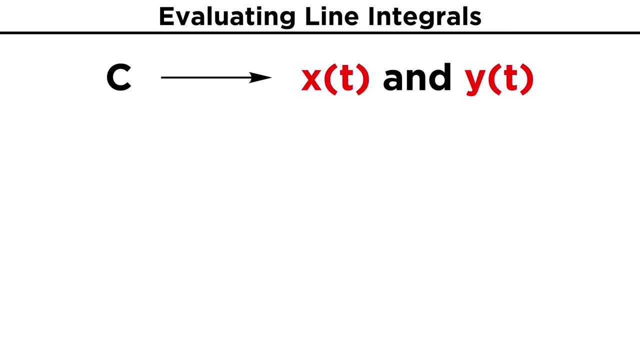 the curve C as two separate equations, one for x and one for y. So let's take a look at line integrals. Let's take a look at line integrals. As we have learned in a previous tutorial, x and y are referred to as parametric. 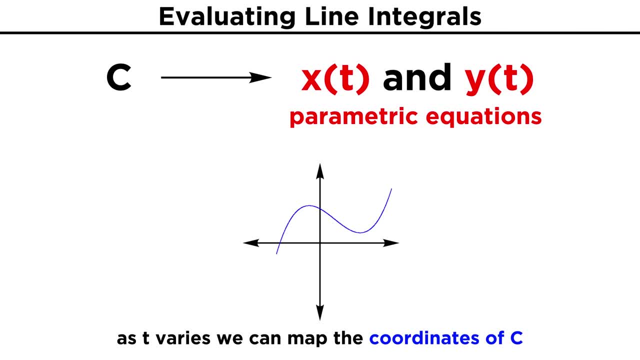 equations and as t varies, the x and y coordinates of the curve they form will be mapped out. For a quick example, consider the equations: x of t equals t over 2, and y of t equals t squared. We can easily see the curve this would map out by solving for t in terms of x and substituting 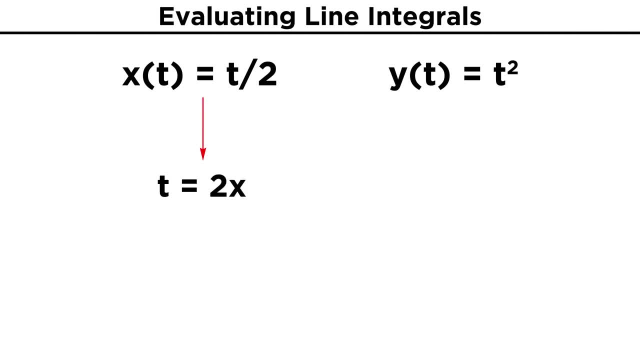 it into the equation for y. By multiplying the first equation by two, we see that t equals two x, which, when plugged into the second equation, gives us y equals two x quantity squared or just four x squared. We can easily plot this equation. 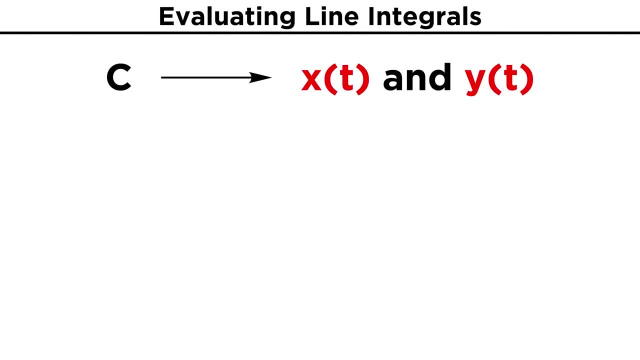 the curve C as two separate equations, one for x and one for y. So let's take a look at line integrals. Let's take a look at line integrals. So let's first break down line integrals. A line around line integrals. Mitarbeiter of line integrals. 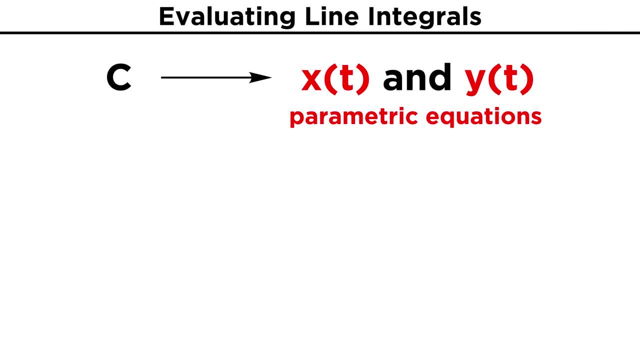 A line around line integrals. A line around line integrals That both depend on a new variable, t. As we have learnt in a previous tutorial, x of t and y of t are referred to as barometric equations and, as t varies, the x and y coordinates of the curve they form will be mapped out. 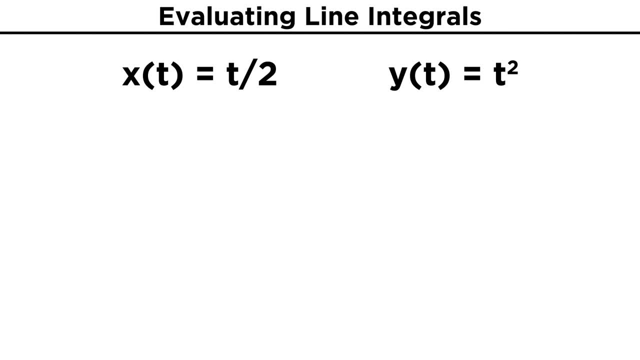 For a quick example, consider the equations x of t equals t over 2, and y of t equals t squared. We can easily see the curve this would map out by solving for t in terms of x and substituting it into the equation for y. 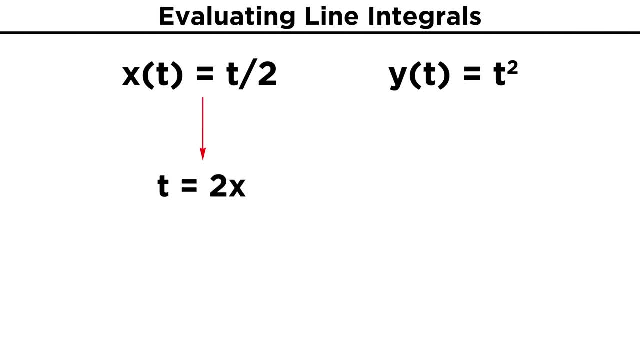 By multiplying the first equation by two, we see that t equals two x, which, when plugged into the second equation, gives us y equals two x, quantity squared, or just four x squared. We can easily plot this equation. Now, let's say t runs from zero to six. 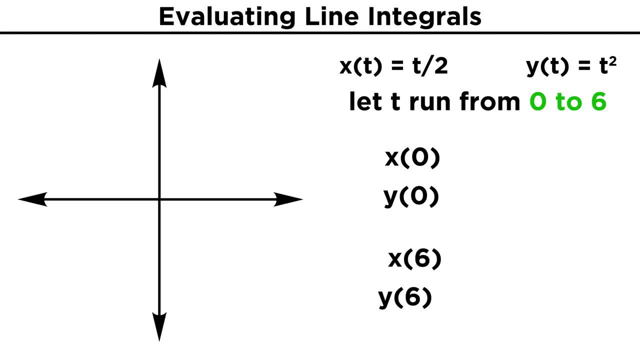 We could plug these values into our parametric equations to get the starting and ending points on this curve for these values of t: For t equals zero, we get x equals zero and y equals zero. For t equals six, we get x equals three and y equals thirty-six. 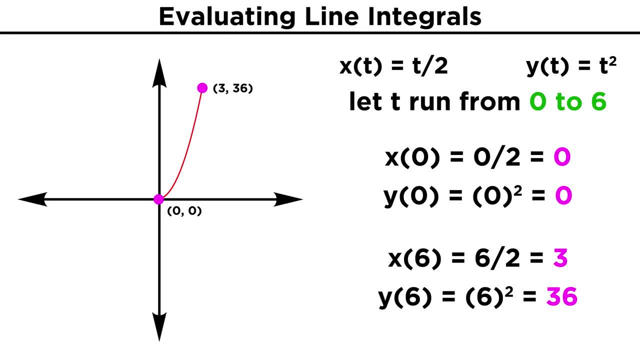 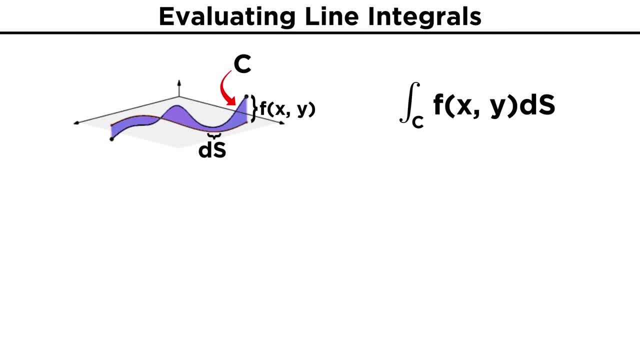 For this range of t. we are left with this part of the curve between these two points. Now why are parametric equations so useful for line integrals? With parametric equations, we can write out the ds term in the integral as something we 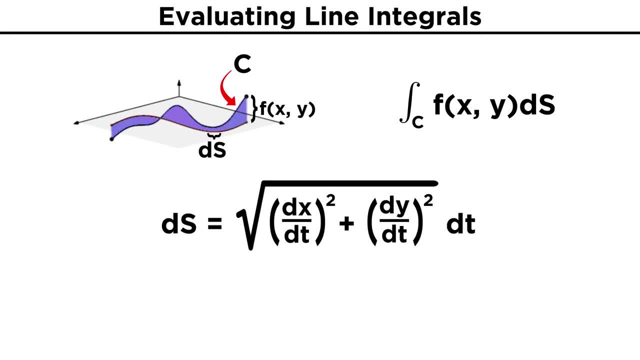 can actually calculate by hand. So ds ends up being equal to root dx. dt squared plus dy, dt squared dt. This represents the infinitesimal space between two points along the curve C, With an incremental change to the parametric variable t. Now that we know this and our integration is in terms of t, we can now express our line. 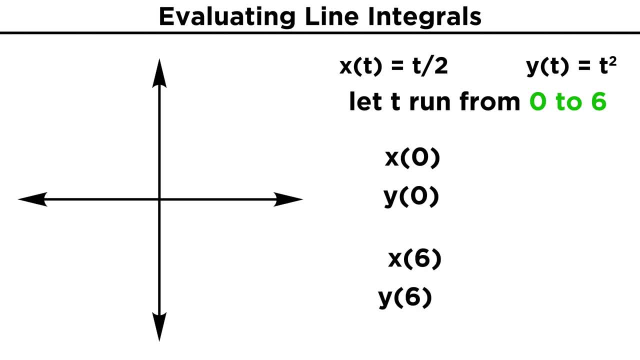 Now let's say t runs from zero to six. We could plug these values into our parametric equations to get the starting and ending points on this curve for these values of t. For t equals zero, we get x equals zero and y equals zero. 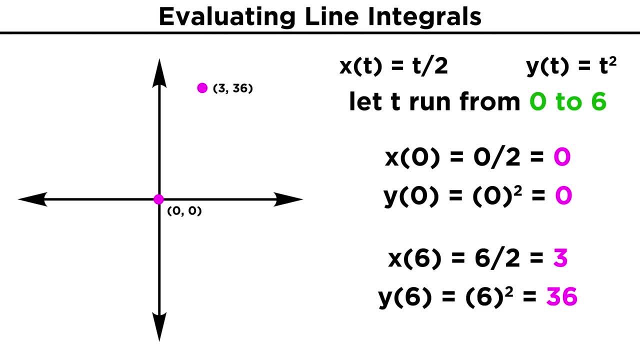 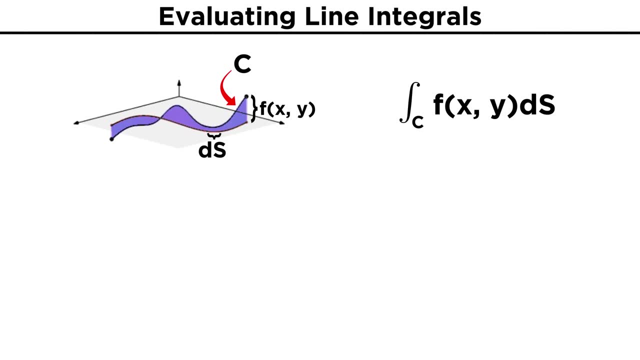 For t equals six, we get x equals three and y equals thirty-six. For this range of t, we are left with this part of the curve between these two points. Now why are parametric equations so useful for line integrals? With parametric equations, we can write out the ds term in the integral as something we 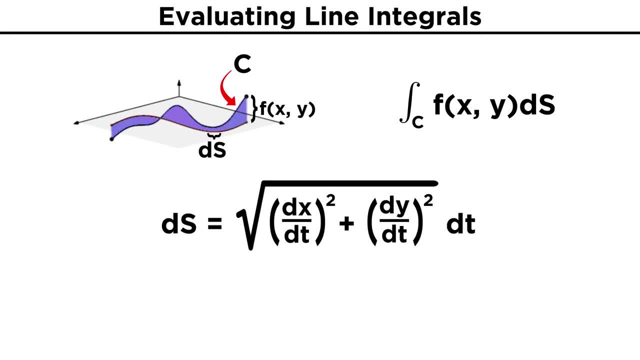 can actually calculate by hand. So ds ends up being equal to root dx. dt squared plus dy, dt squared dt. This represents the infinitesimal space between two points along the curve C, With an incremental change to the parametric variable t. Now that we know this and our integration is in terms of t, we can now express our line. 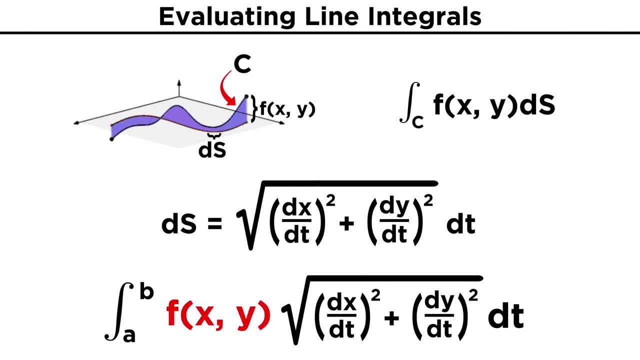 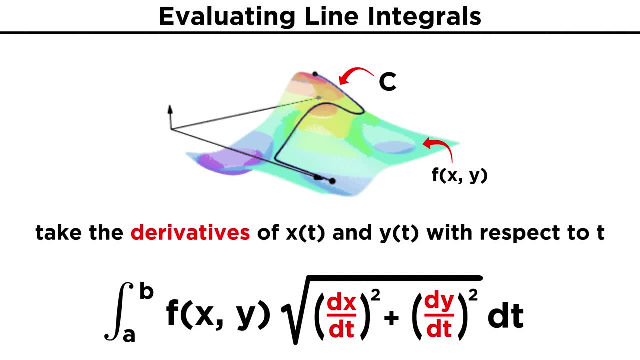 integral as the integral from A to B of f root dx dt squared plus dy dt squared dt. So, given a surface f and a curve C, we must take the derivatives of the parametric equations with respect to t and plug everything into this equation. 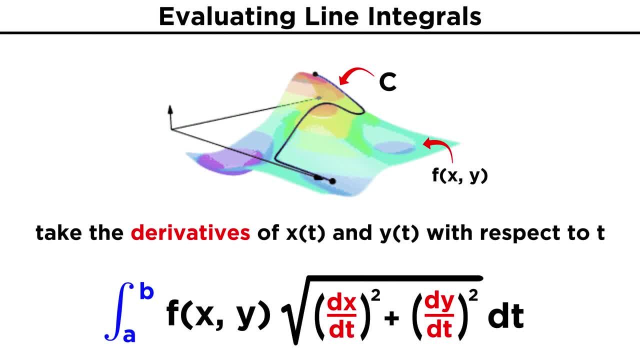 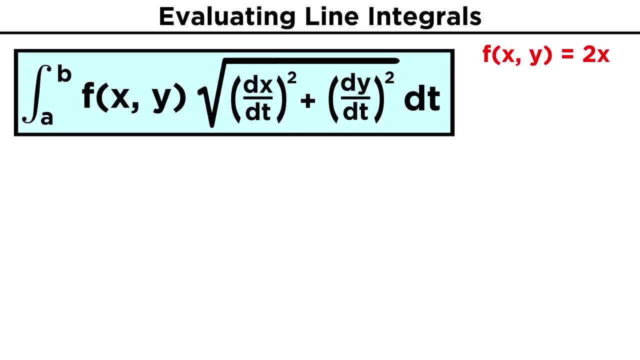 Then we integrate from the lower bound of t, which is A, to the upper bound of t, which is B. As an example, consider the surface given by f of x. y equals two x and our curve, C, being the same as the one we discussed earlier. with parametric equations, x of t equals t. 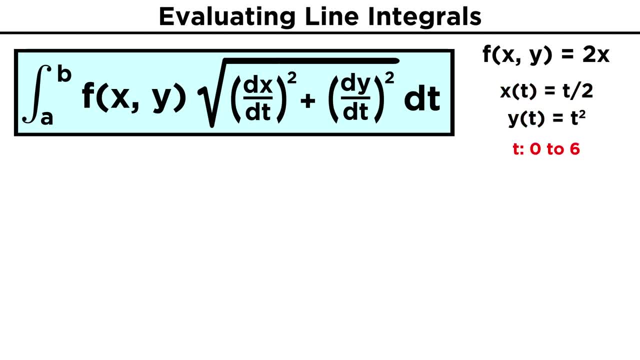 over two And y of t equals t squared, letting t run from zero to six. We can go ahead and plug all of this information into our equation for line integrals, But notice that f of x- y is still in terms of x, whereas we want to integrate with respect. 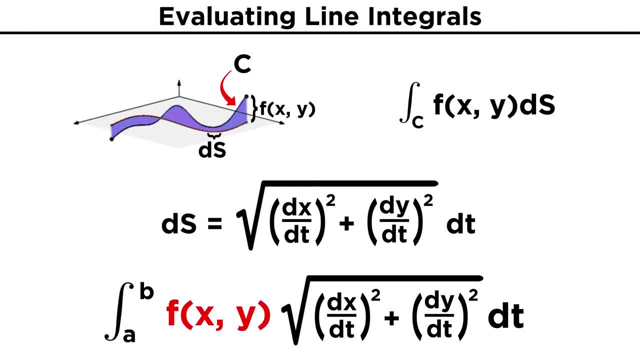 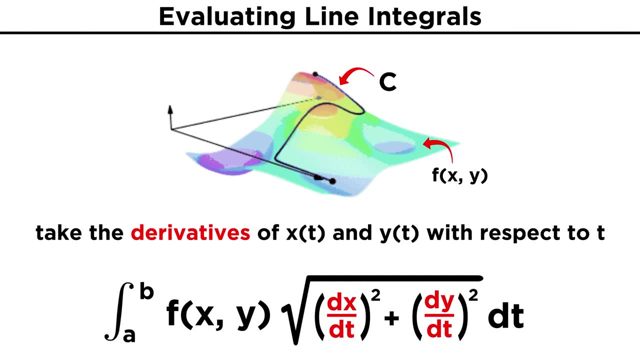 integral as the integral from A to B of f root dx dt squared plus dy dt squared dt. So, given a surface f and a curve C, we must take the derivatives of the parametric equation with respect to t and plug everything into this equation. 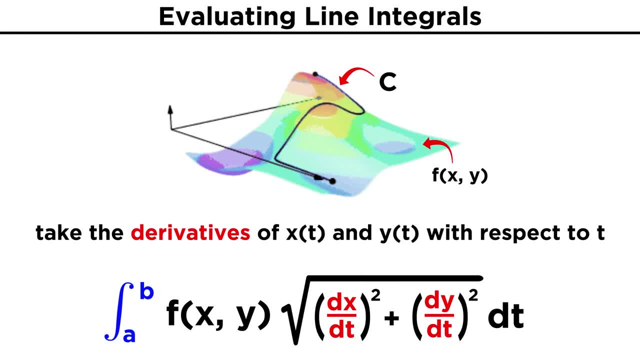 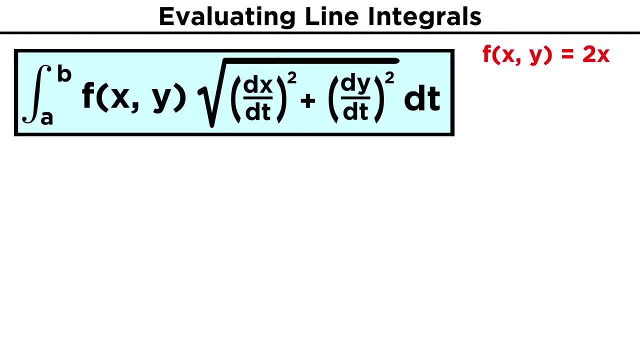 Then we integrate from the lower bound of t, which is A, to the upper bound of t, which is B. As an example, consider the surface given by f of xy equals two x and our curve, C, being the same as the one we discussed earlier. with parametric equations, x of t equals t over. 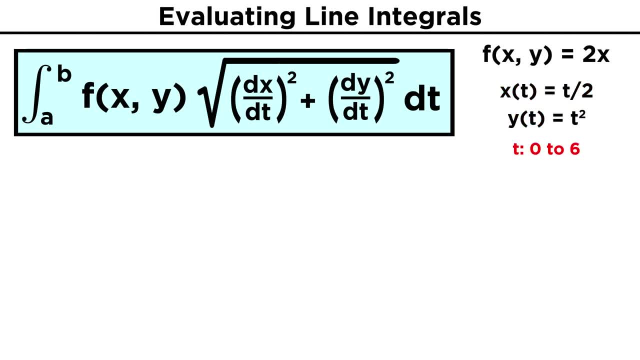 two and y of x equals zero, t equals t squared, letting t run from zero to six. We can go ahead and plug all of this information into our equation for line integrals, but notice that f is still in terms of x, whereas we want to integrate with respect. 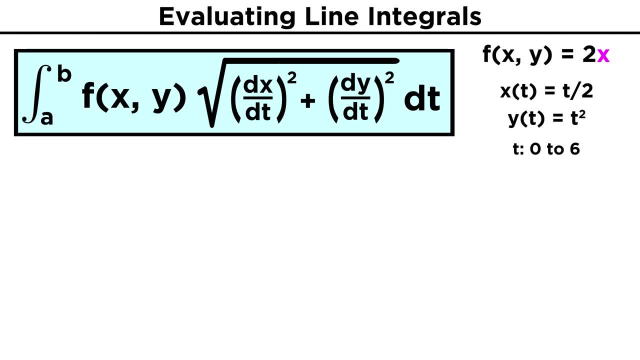 to t, We must replace the x with the appropriate expression in terms of t. Luckily, the parametric equation x of t gives us just that, so we can replace x with t over two. Now we must get the terms dx, dt and dy dt, which will just be the derivatives of the. 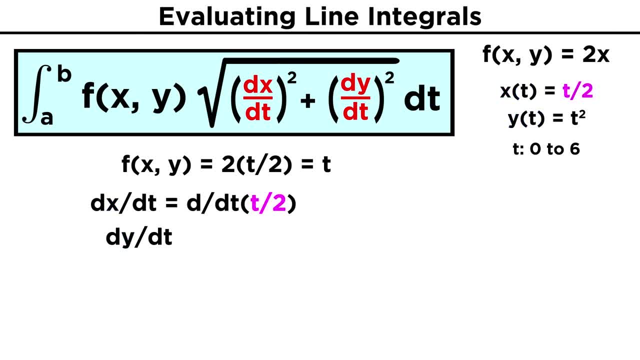 parametric equations: Differentiating x of t equals t over two, we get dx dt equals one half. and for y of t equals t squared, we get dy dt equals one half. Plugging everything in our line integral becomes the integral from zero to six of t. 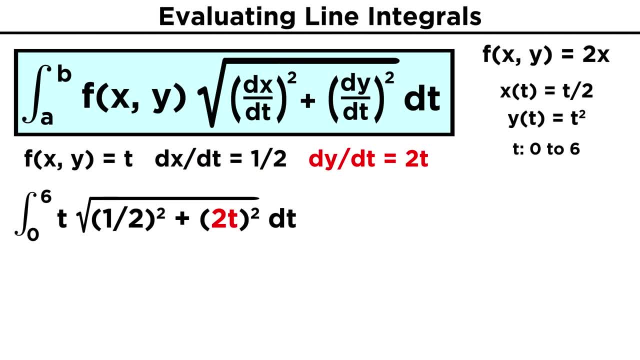 root one half squared plus two t, quantity squared dt, which simplifies to the integral of t root one fourth plus four t squared dt. To solve this we must use substitution, letting u equal one fourth plus two t, So we can get this right. 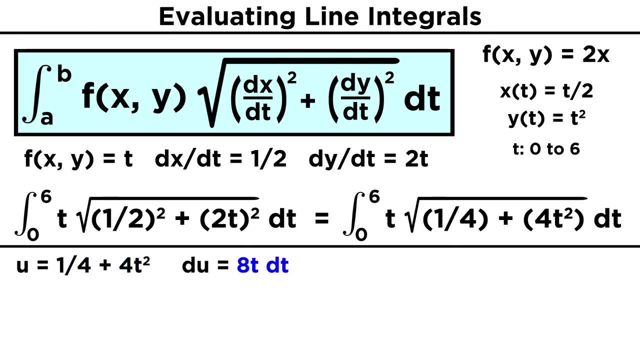 Let's do the next expression. Let's do it: 1 plus 1 is equal to two t plus four t squared, which, when we differentiate both sides, gives du equals eight t dt. We have t? dt in the expression, so let's change that to du over eight. 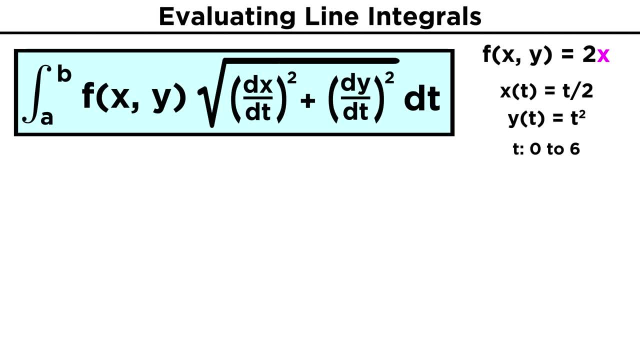 to t, We must replace the x with the appropriate expression in terms of t. Luckily, the parametric equation x of t gives us just that, So we can replace x with t over two. Now we must get the terms dx, dt and dy dt, which will just be the derivatives of the. 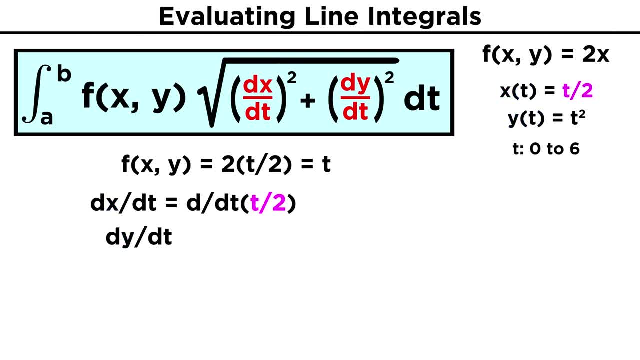 parametric equations: Differentiating x of t equals t over two, we get dx. dt equals one half, and for y of t equals t squared, we get dy dt equals two t. Plugging everything in our line integral becomes the integral from zero to six of t. 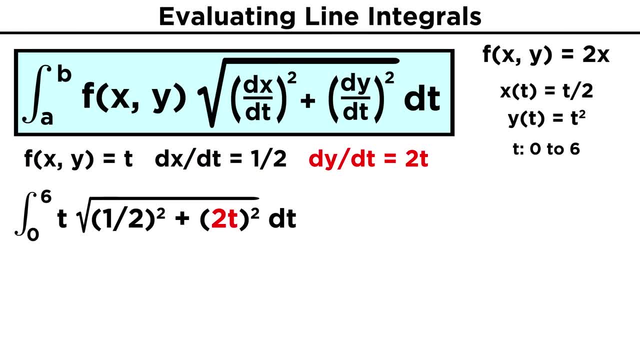 root one half squared plus two t quantity squared dt, which simplifies to the integral of t root one fourth plus four t squared dt. To solve this we must use substitution letting u equal one fourth plus four t squared which, when we differentiate both sides, gives du equals eight t dt. 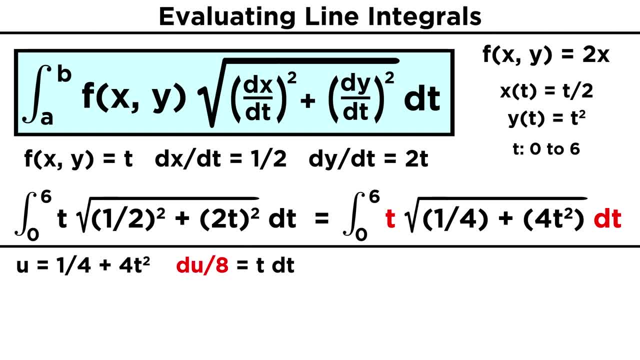 We have t dt in the expression, so let's change that to du over eight. And now we can write the line integral strictly in terms of u, which gives us one eighth times the integral of root, u, du. This is simple to integrate if we think of the root as an exponent equal to one half. 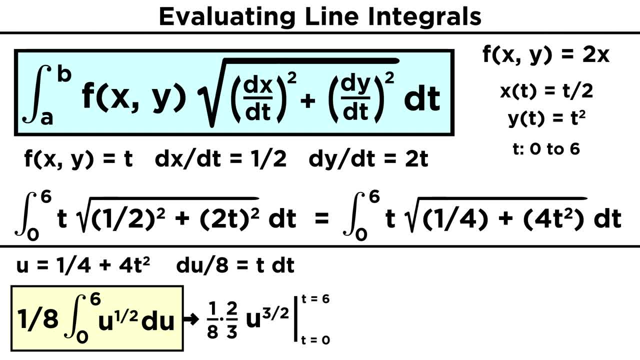 We will get one eighth times two thirds u to the three halves evaluated from the lower bound of zero to the upper bound of six. Simplifying and plugging our original expression back in, we have one twelfth times one fourth plus four t squared to the three halves from zero to six. 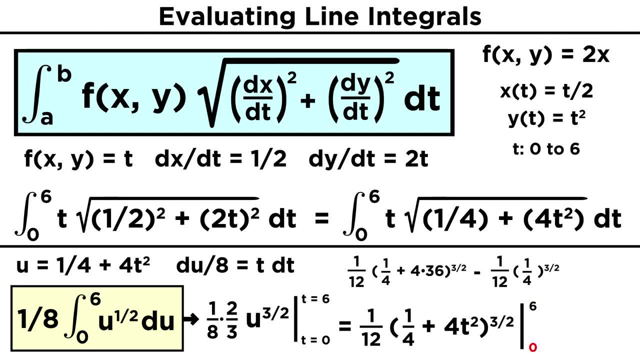 Plugging in t equals six, and subtracting from that the expression at t equals zero. we get one twelfth times one fourth plus four times thirty-six to the three halves, minus one twelfth times one fourth to the three halves. Plugging this into a calculator gives us approximately one hundred forty-four point three six. 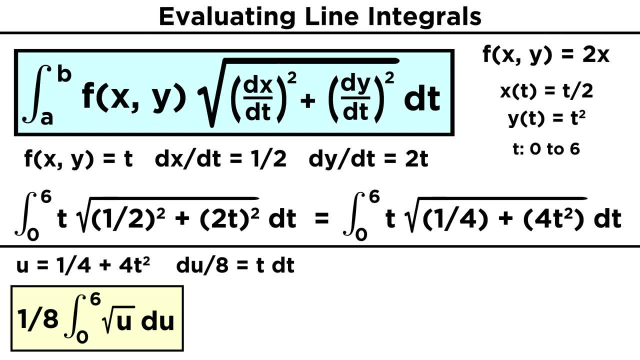 And now we can write the line integral strictly in terms of u, which gives us one eighth times the integral of root u, du. This is simple to integrate. if we think of the root as an exponent equal to one half, We will get one eighth times two thirds u to the three halves evaluated from the lower. 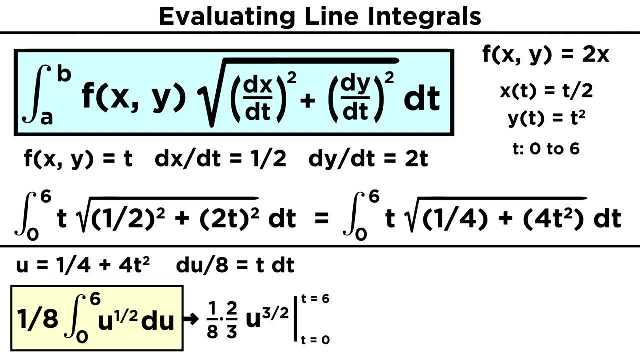 bound of zero to the upper bound of six. Simplifying and plugging our original expression back in, we have one twelfth times one, fourth plus four t squared to the three halves from zero to six. Putting in t equals six and subtracting from that the expression at t equals zero. 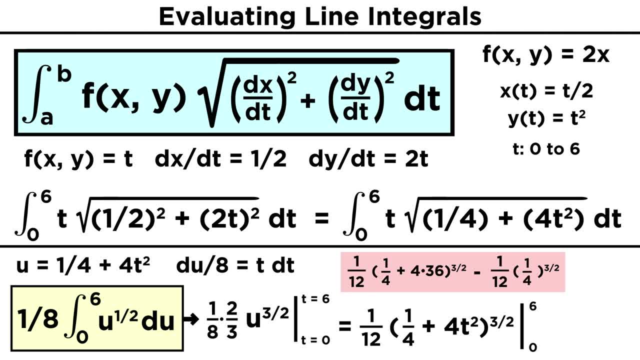 we get one twelfth times one fourth plus four times thirty-six to the three halves, minus one twelfth times one fourth to the three halves. Plugging this into a calculator gives us approximately one hundred forty-four point three six. This is the area under the surface. f of x. y equals two x along our curve, which is: 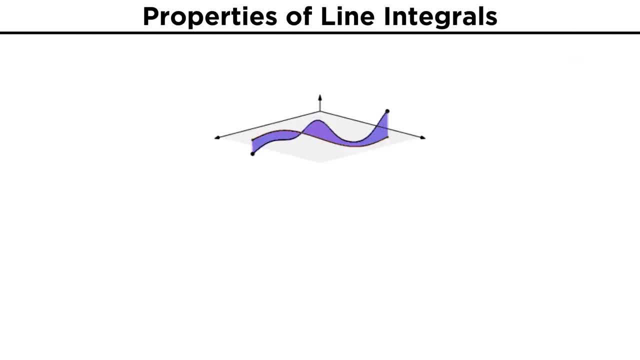 c. We have now gone over the basic approach for line integrals, but like many concepts in math, their applications and complexity can vary. A useful property for more complex cases is the ability to split a curve up into separate pieces for integration. Given a curve like this, for example, you could consider each part of it as separate curves. 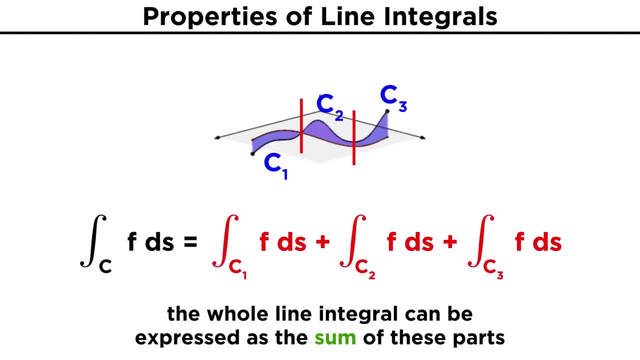 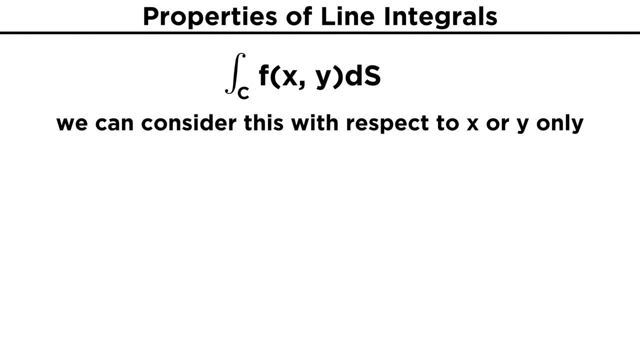 and the whole line integral can be expressed as the sum of each. It's also possible to consider line integrals with respect to x and y. only, These are much simpler calculations, as the ds is simply replaced with dx or dy respectively, And if we want to put these in parametric form, we get the integral from a to b of f. 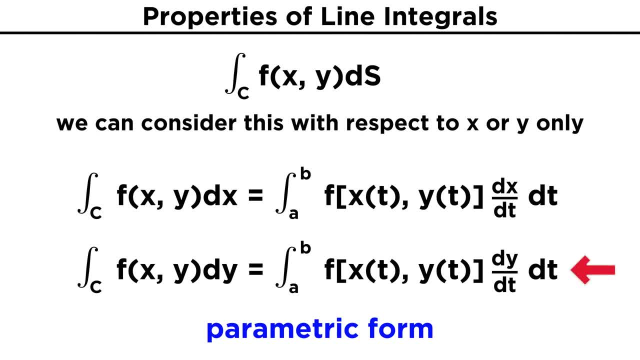 dx, dt, dt for x and the integral from a to b of f dy, dt, dt for y. So that leaves us with the famous integral of a to b of f dx, dt, dt for x and the integral from a to b of f dy, dt, dt for y. 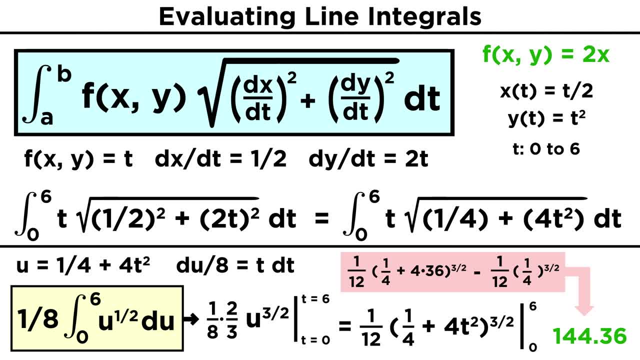 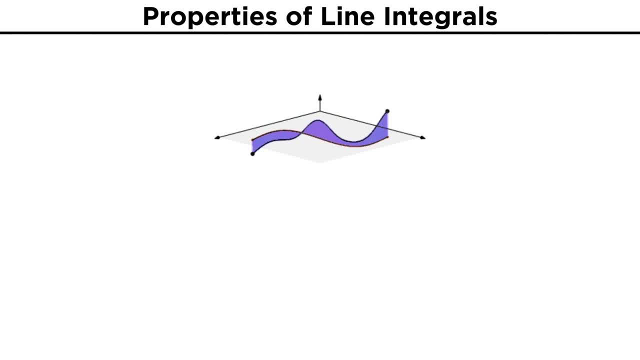 This is the area under the surface f of x. y equals two x along our curve C. We have now gone over the basic approach for line integrals, But like many concepts in math, their applications and complexity can vary. A useful property for more complex cases is the ability to split a curve up into separate 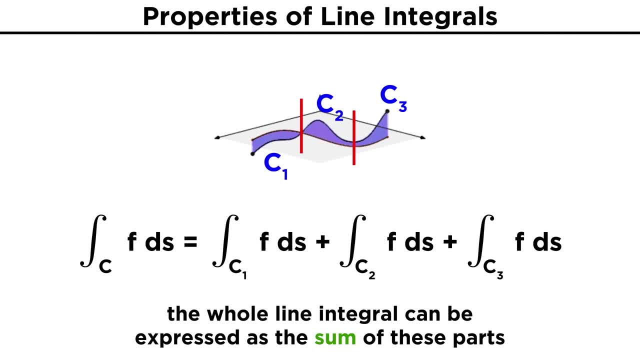 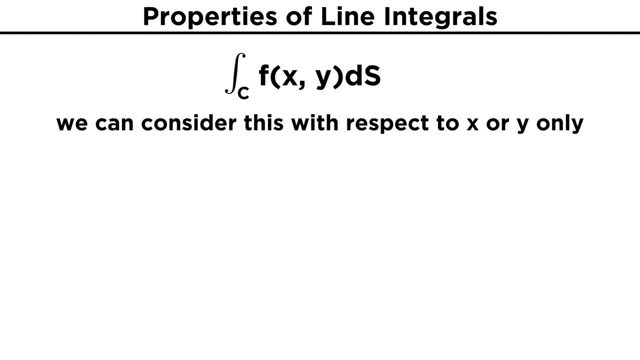 pieces for integration. Given a curve like this, for example, you could consider each part of it as separate curves and the whole line integral can be expressed as the sum of each. It's also possible to consider line integrals with respect to x and y. 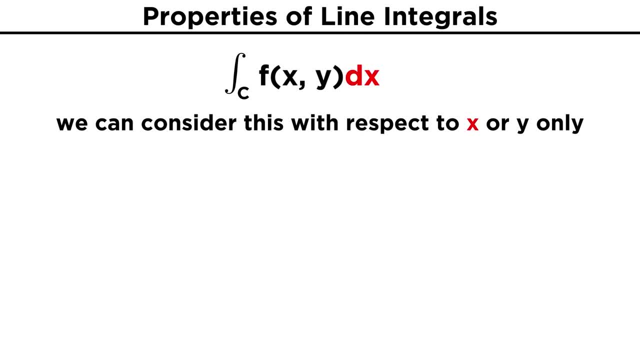 These are much simpler calculations, as the ds is simply replaced with dx or dy respectively, And if we want to put these in parametric form, we get the integral from A to B of f, dx, dt, dt for x and the integral from A to B of f, dy, dt, dt for y. 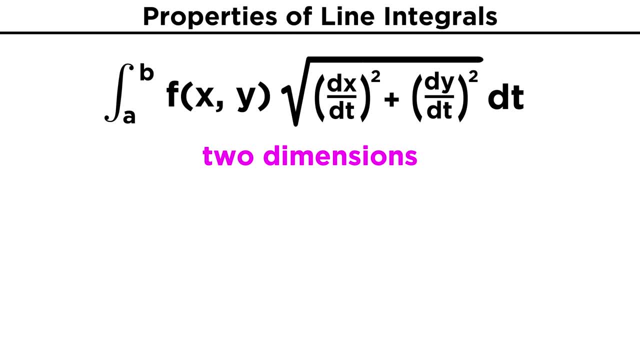 One more thing to note is that line integrals are not limited to just line integrals. They are not limited to just line integrals. They are not limited to just line integrals. They are not limited to just the dimensions we have been using here. 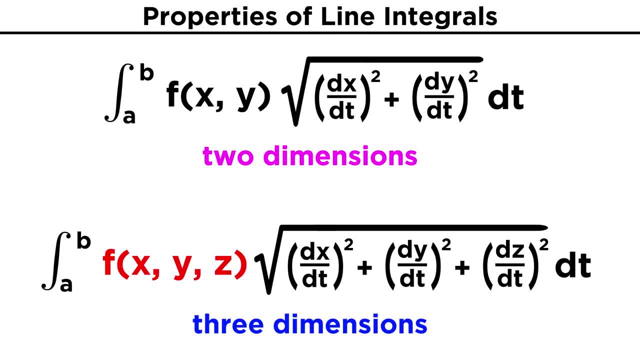 If we wanted a line integral of a function f, we would need to use a higher dimensional ds, which ends up being root dx, dt squared plus dy, dt squared plus dz, dt squared- dt. Additionally, line integrals become very useful with vector fields. 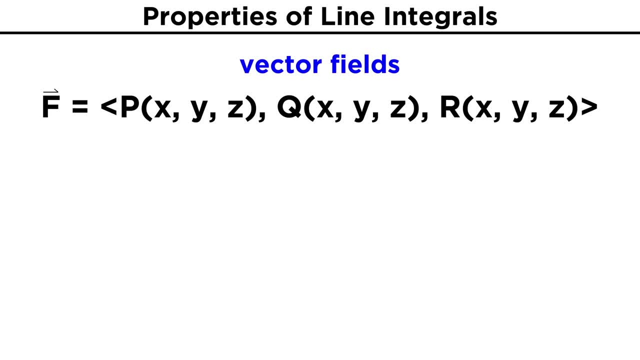 Recall that vector fields have the form f and the vector fields have the form orc. so we don't need to 요k with Bh into f, del, n, orc. but from the view of the general form we can say that if f, animal re, Jenny, stay zero, orc, an integral that Mitur or. 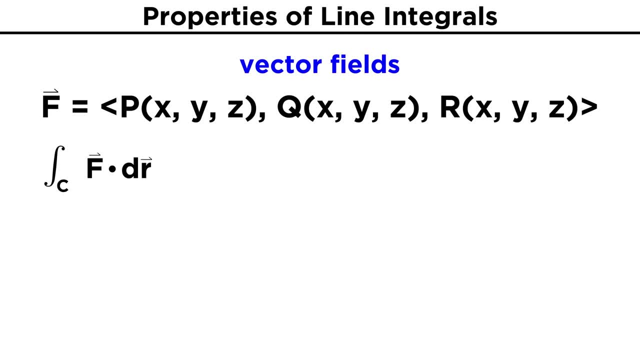 be z equal to x perλ. the integral ofiskd d without Haj frx be long 3a, dEız, x e, SW. The line integral of this vector field along some curve, C is given by the integral along c of f, dot, dr, where dr is the vector, dx dy. 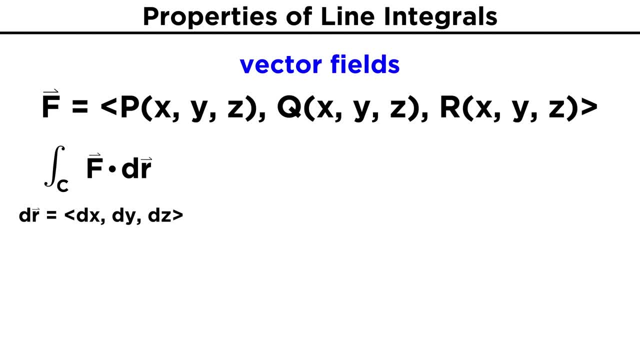 dz. Going through the dot product we can see that the ending integral can be expressed as the integral over c of p, dx plus q, dy plus 4x, dx plus 5y, z times y for the spirit sinusнения are dz. 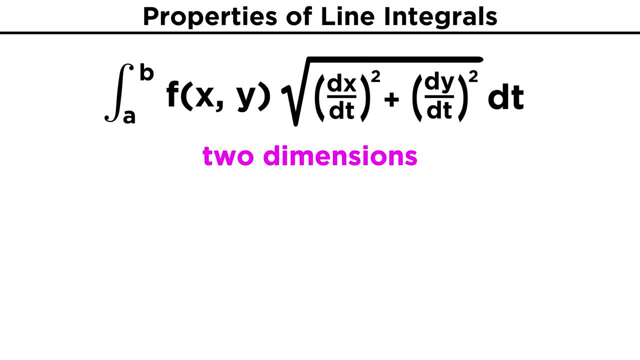 One more thing to note is that line integrals are not limited to just the dimensions we have been using here. If we wanted a line integral of a function f, we would need to use a higher dimensional ds, which ends up being root dx- dt squared plus dy- dt squared plus dz- dt squared. 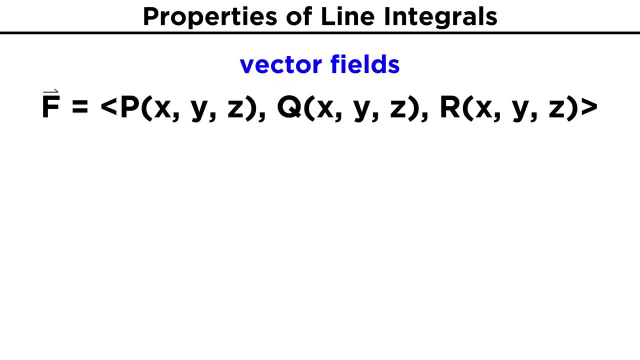 dt. Additionally, line integrals become very useful with vector fields. Recall that vector fields have the form f equals pxyz, qxyz, rxyz. The line integral of this vector field along some curve, C, is given by the integral along C of f, dot, dr, where dr is the vector, dxdydz. 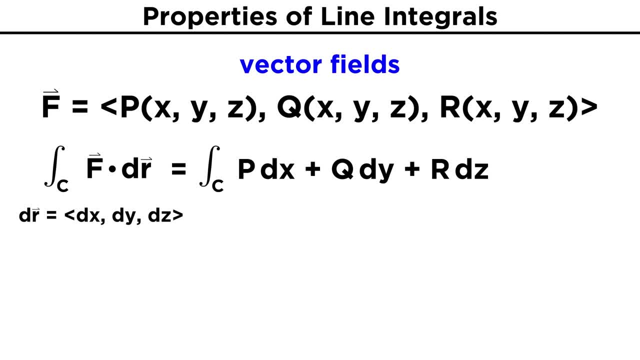 Going through the dot product, we can see that the line integral can be expressed as the integral over C of pdx plus qdy plus rdz. If our curve is parameterized by t, the dx can be replaced with dxdtdt, the dy by dydtdt. 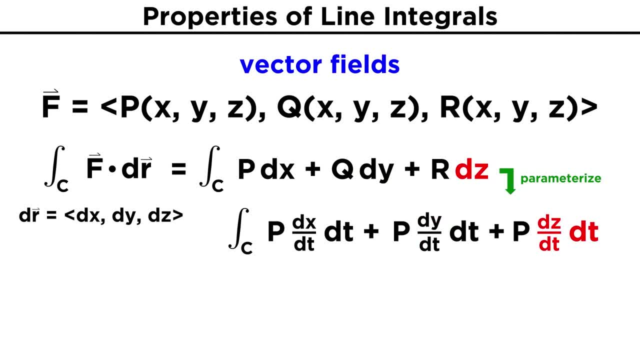 and the dz by dzdtdt. What this line integration calculates with vector fields can be thought of as how we know how much of the vector field is in the direction of the curve. This makes sense as we are dotting the vector field which takes the tangential component. 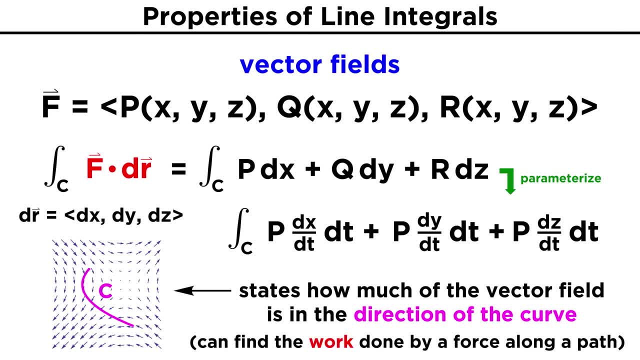 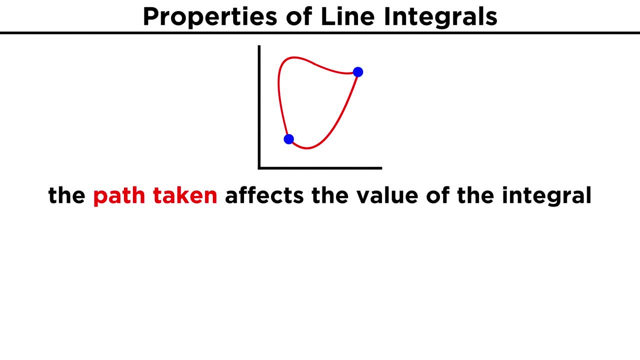 of the field to the path of the curve. In physics, this calculation can be used to find the work done by a force along a path. An important thing to note about line integrals is that in most cases, the path taken affects the answer. 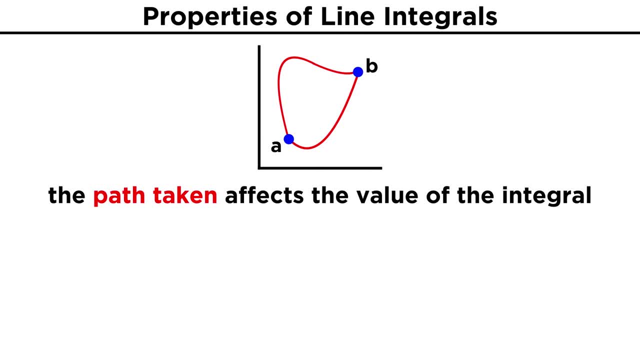 That is, even with the same starting and ending points A and B, the line integral over different paths can yield different answers. There is an exception that will cause line integrals to be independent of paths, and this is when the vector field f is conservative. 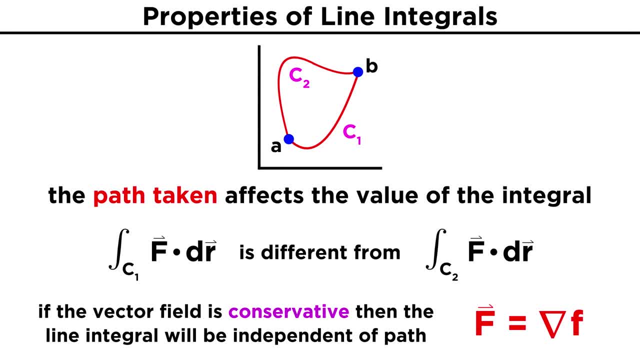 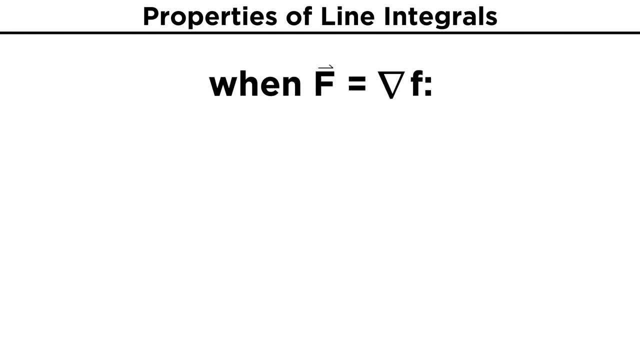 Remember. this means that the vector field can be written as the gradient of some function f Here Think again. This is because the line integrals of gradient, which is the gradient of some function f, gradient vectors- have a special property to them. 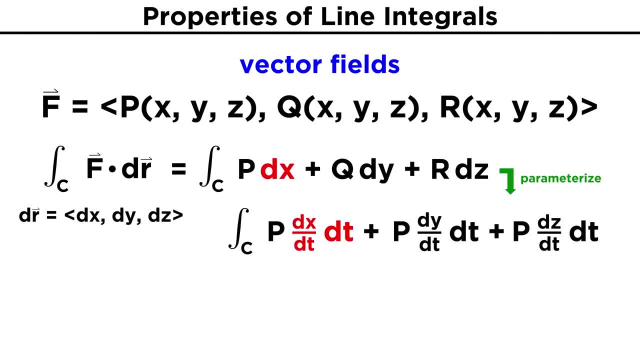 If our curve is parameterized by t, the dx can be replaced with dx, dt, dt, the dy by dy, dt, dt and the dz by dz, dt, dt. What this line integration calculates with vector fields can be thought of as how much of the vector field is in the direction of the curve. 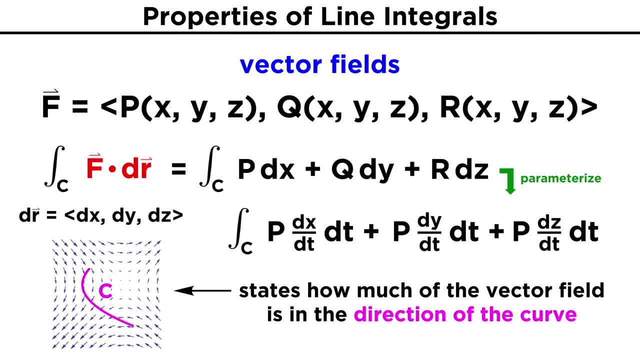 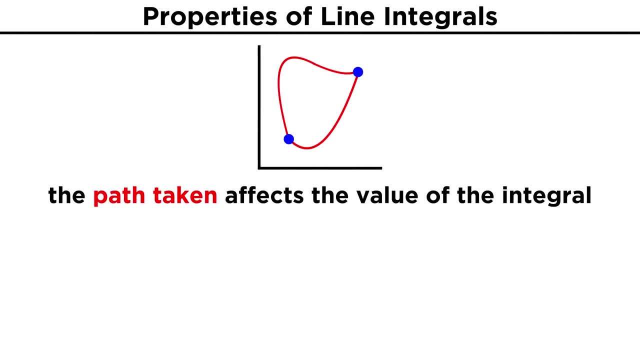 This makes sense as we are dotting the vector field, which takes the tangential component of the field, to the path of the curve. In physics, this calculation can be used to find the work done by a force along a path. An important thing to note about line integrals is that in most cases, the path taken affects. 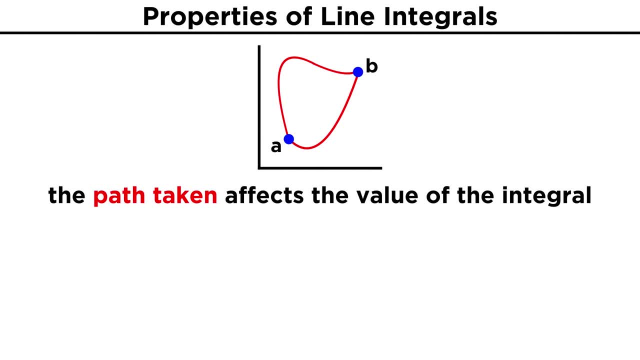 the answer. That is, even with the same starting and ending points A and B- the line integral over d. different paths can yield different answers. There is an exception that will cause line integrals to be independent of paths, and this is when the vector field F is conservative. 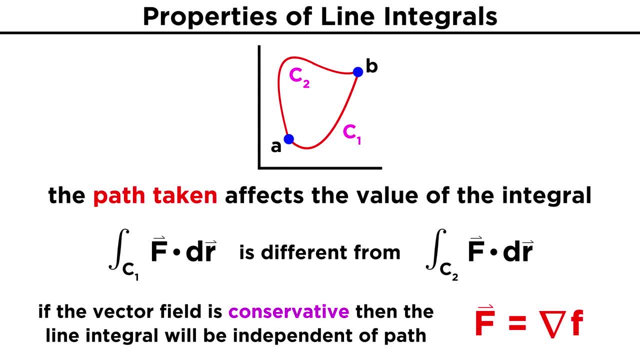 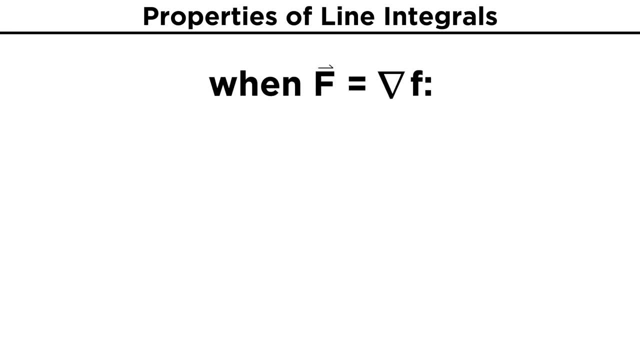 Remember this means that the vector field can be written as the gradient of some function F. This is because the line integrals of gradient vectors have a special property to them. The integral over a curve C of a certain function F is a linear function. This is how we know a vector field is conservative. We can use the line integrals to solve different questions for this exam. So let's see how to solve an equation called the linear equation. Let's see how to solve an equation called the linear equation. 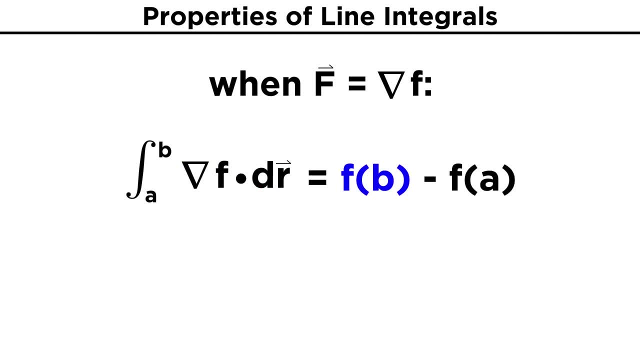 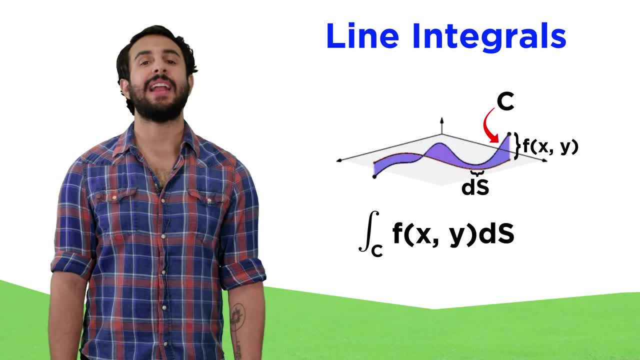 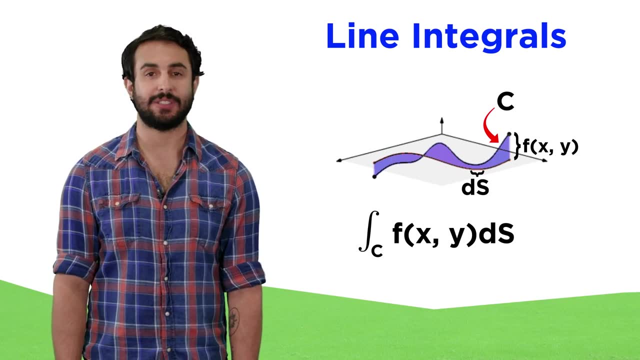 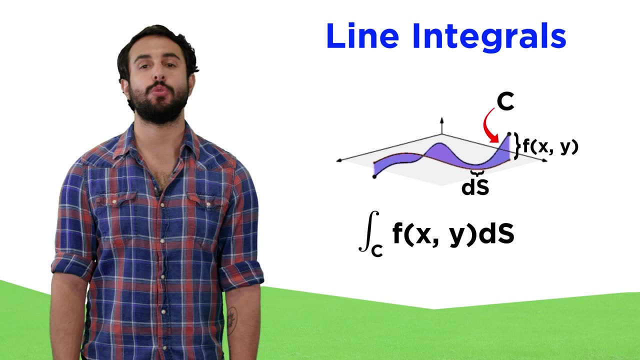 line integrals. Line integrals can be a bit confusing due to the notation and having to take the curves into account for calculations, but we have outlined a range of uses and this will be important in understanding a theorem which we will be discussing soon.